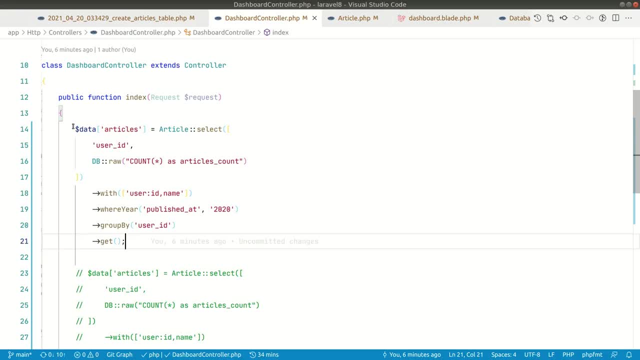 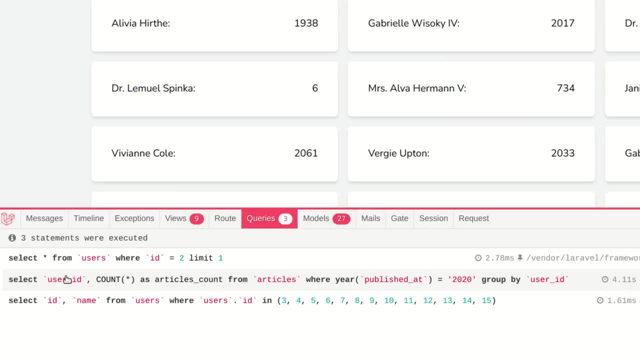 query that we are looking here. so this one is the query that is being run from here and, as you can see here, it is taking about 4.11 seconds and you can see here it is doing select user id and the count as articles count from articles where published at date is this year. 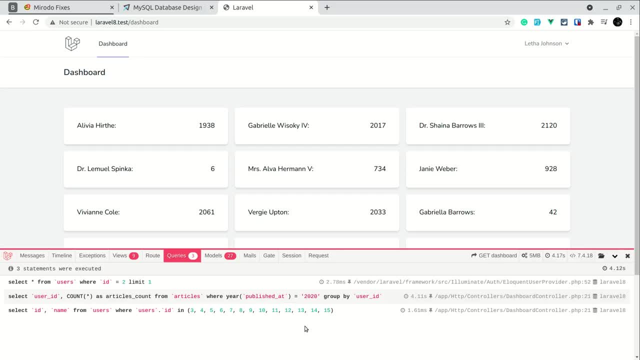 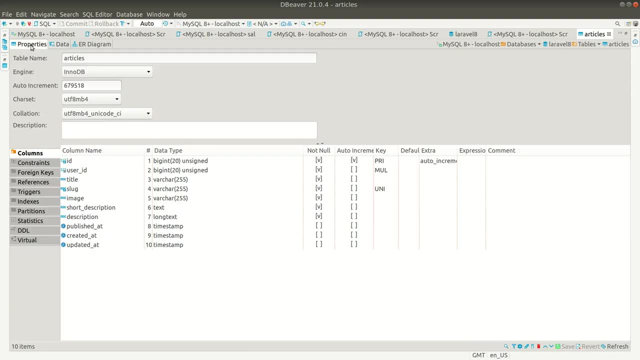 is 2020 and it is grouping all by user id. so you can see here, guys, it is taking about 4.11 seconds and if we look here in the database, the articles, the properties, so it has these data here. and if we look here in the indexes, it has some indexes, but also it is not doing any. 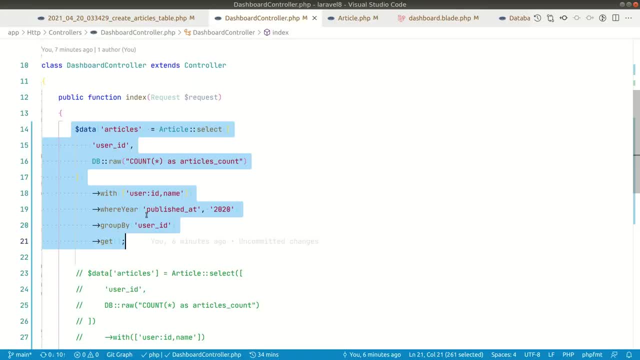 trick why? let's see. so if you see here we are just doing where condition on published at. basically, in order to make a query very much faster, you need to put an index on the column by which you are querying. so currently we are querying here using the published ad. 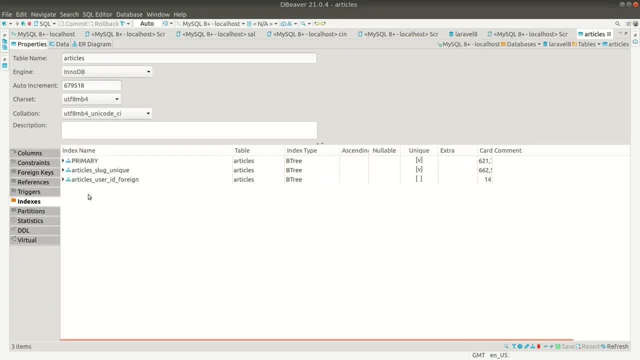 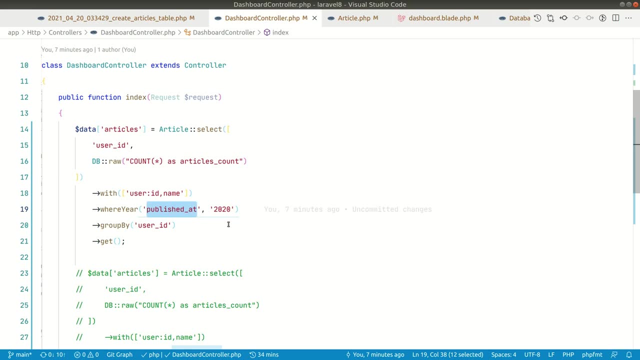 date where published ad date. but in our this database we don't have any index on the published at column. so let's try to add the query on the published at column and let's see whether it makes a difference or not. so we can do that using laravel migration. so let's do that, create a migration. 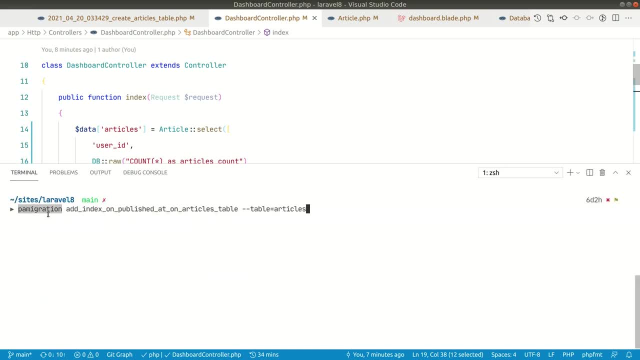 so this pa migration is just a shortcut for php artisan make migration. this is an alias i have created now add index on published ad column. so i have written this as an alias because this is an τιangii我很 kort. yirgnirg Rafael's wil 보니. let me show you subscribe and after號 i will. 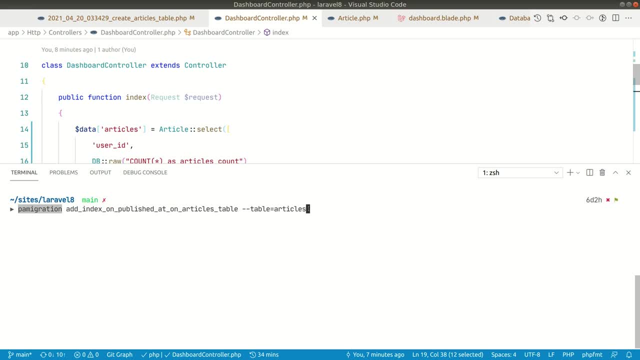 date ob 들어가 pos이다. next slide come with parsingWhich become these columns at date? OMG, now add index on published at articles table and on the articles table so you can give any name. this one, okay. so i have just given specific name so that it will be easier if you look this one in. 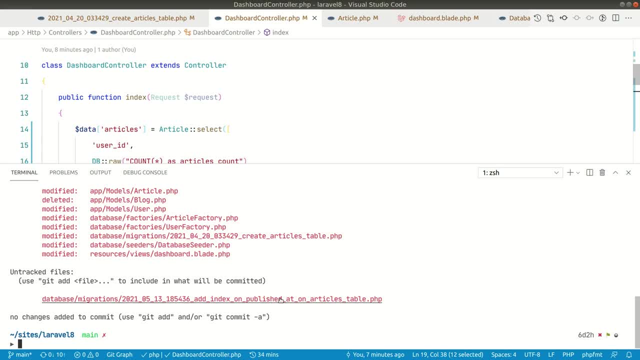 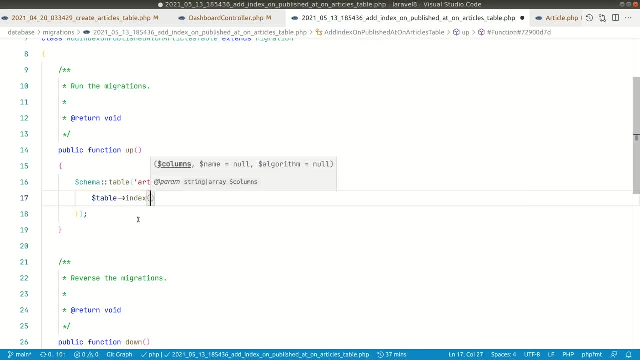 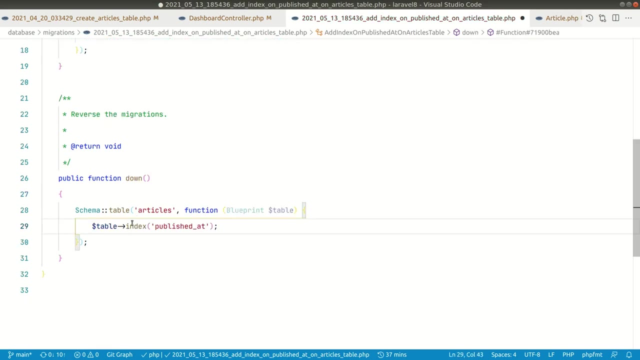 the future. so it is now created. now let me go to the file here. now let us add an index table index to the published at column on the down method. we need to drop the index. so if you, whenever we do a rollback, so it will just do the opposite. we have to add this in: 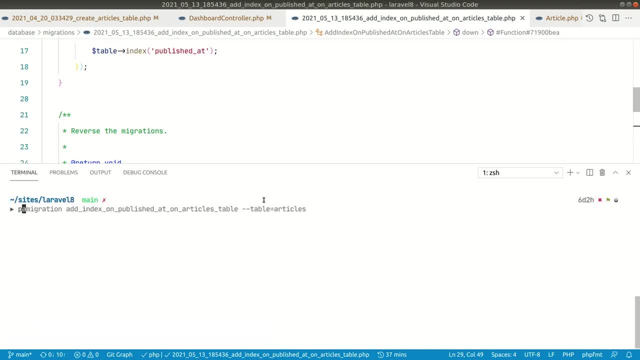 array like this. so now we have done this, now let us run the migration. it will take a little bit while because there are a lot of data currently. the migration has run successfully now if we see here and refresh the page here so you can see here articles published at index. so this index is. 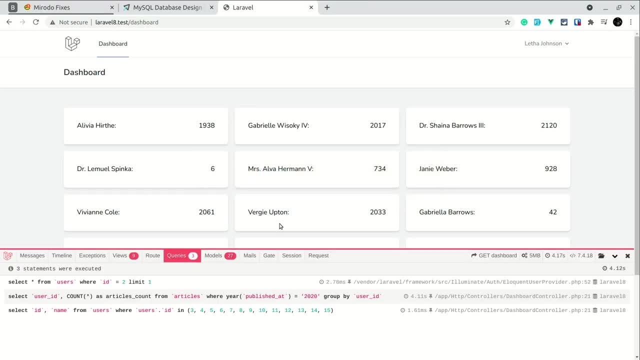 added to the published at now, if we go in the browser and refresh the page, hmm, hmm, hmm, it is again taking a lot of time, guys. so if you see here, it is taking again about 3.8 seconds. hmm, the index did not work, or did it? so if we see here, guys, in our query, in the dashboard controller, 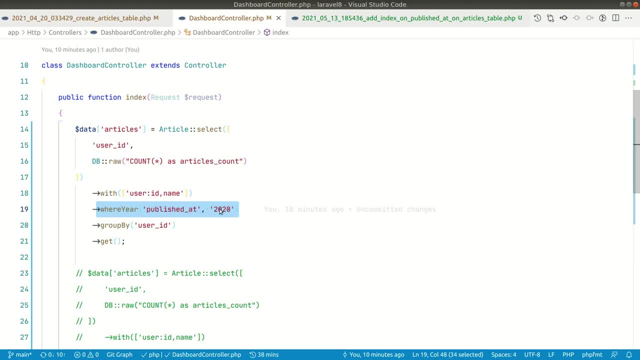 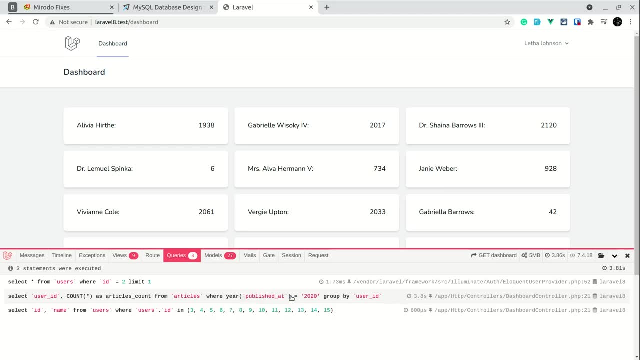 we are doing with year published at. yes, so now, if we look here in the actual query, so it is calling this year published at. so it is just calling a function year where we have passed the published at column as a parameter. so it is not directly using the published at column, so that's. 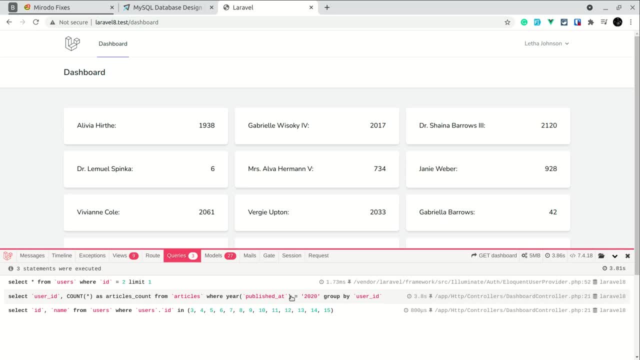 why the index is not working. so, guys, in order to make our query performant, we have to think in a different way, so we can also accomplish the same results using a different queries. now let's see how to do that, and that will be much more faster than this. so it is currently 3.8 second, and let's 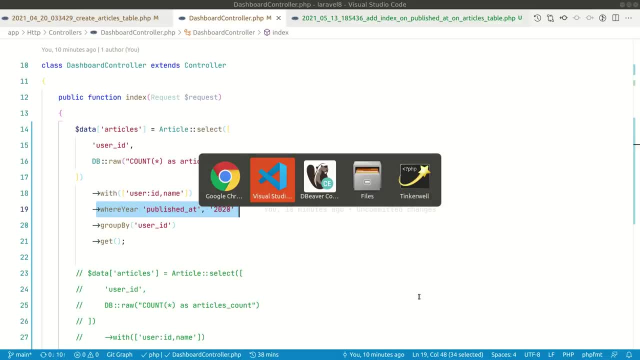 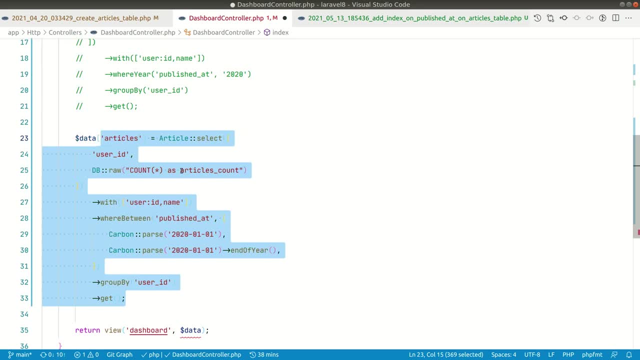 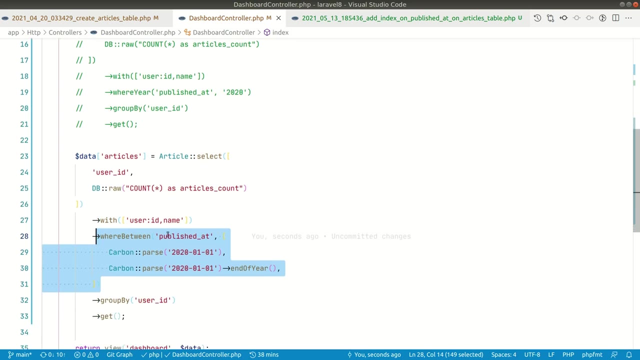 see if we implement it and how much time will it take. now, if I just comment this one, I have already prepared the query, so that, hmm, so let me uncomment this. so if you see, here, guys, everything is same except this one. so select user id and count from the articles and user and published at is where between now instead of 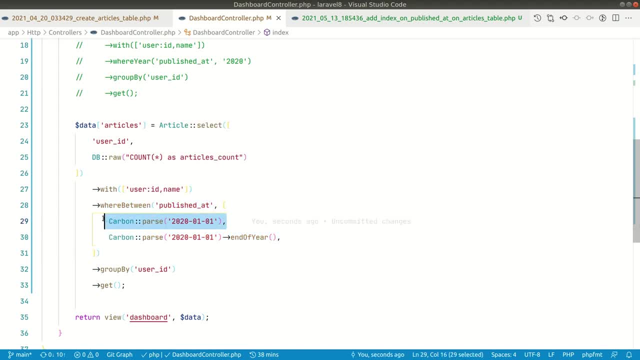 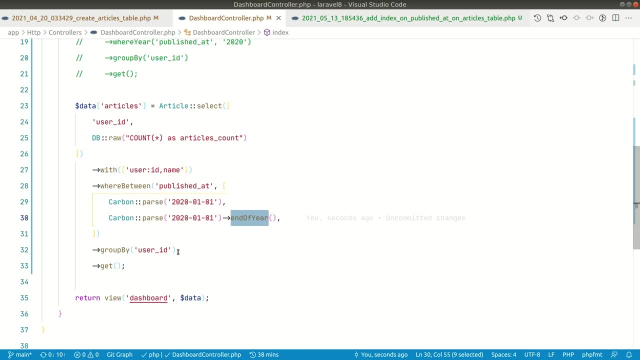 where year we are using, where between, and the start will be 2020, the same year- beginning of the year and 2020 end of the year, and everything other is same. now, if we go here in the browser and refresh the page and you can see here, guys, 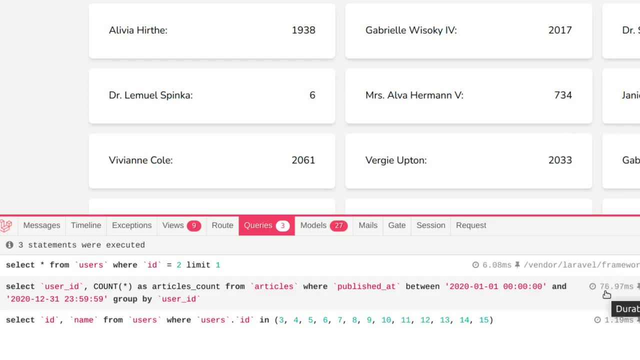 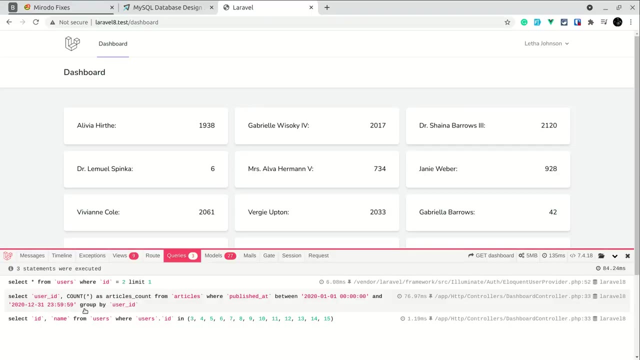 hmm, it is much more faster, which is only 76 milliseconds. so if you look here, the query now this is: there is a different query where published at is between the beginning of the 2020 year and the end of the 2020 year. so just by modifying a query slightly, we can. 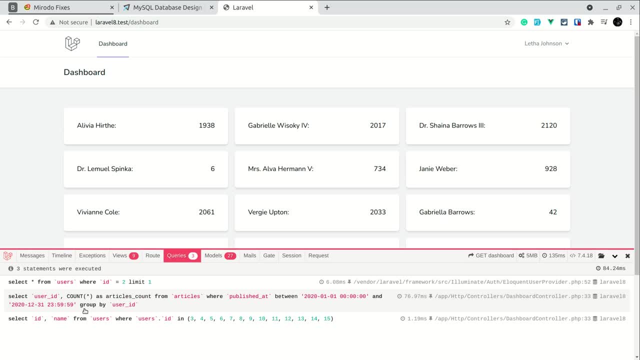 highly increase performance of our query. if you didn't have any index, then using the same query would also take about three to four seconds, but after adding the index the performance of this query increased, so that's something that I can set the same. goodbye to our software in the next statement: just put in couple or adding a few numbers, and we're ready now. so, anyways, let's see how to perform this query. if you didn't have any index, then using the same query would also take about three to four seconds. after adding the index, the performance of this query increased. so now let's see how.